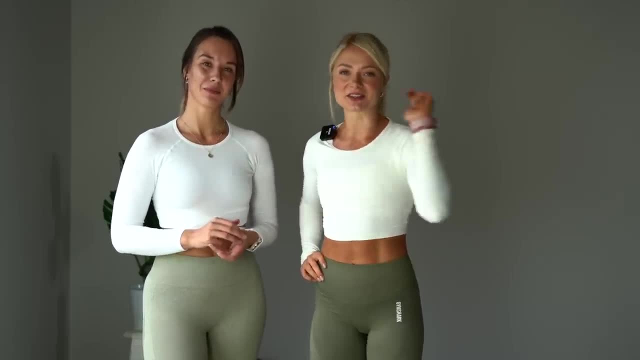 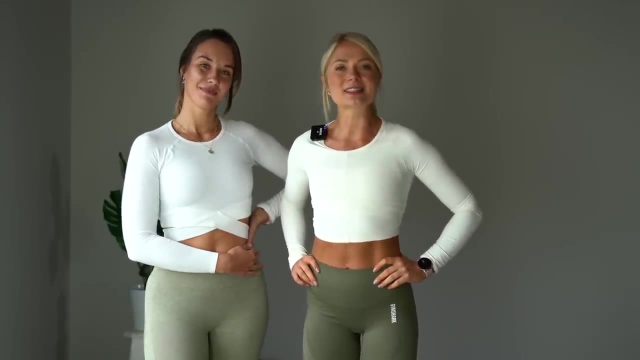 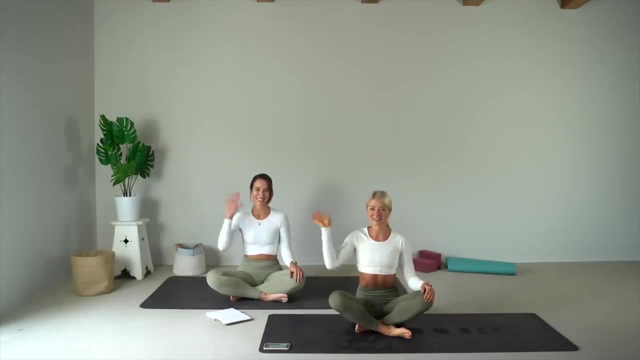 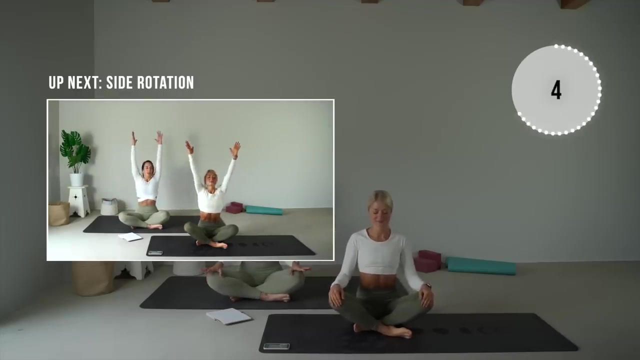 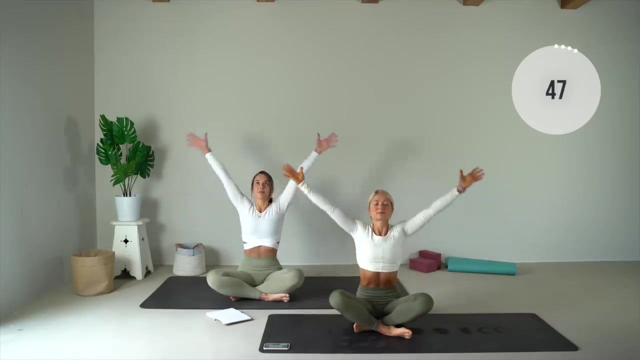 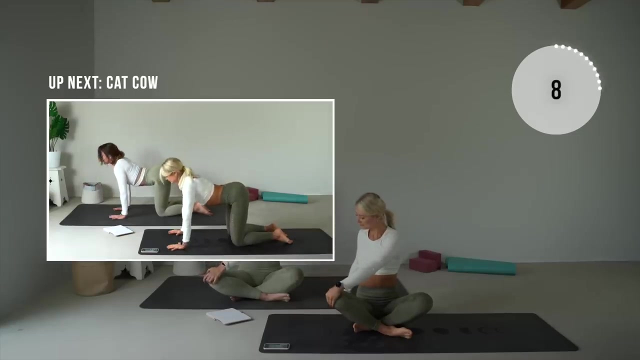 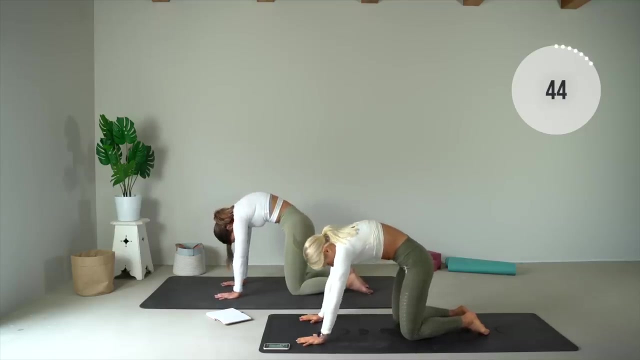 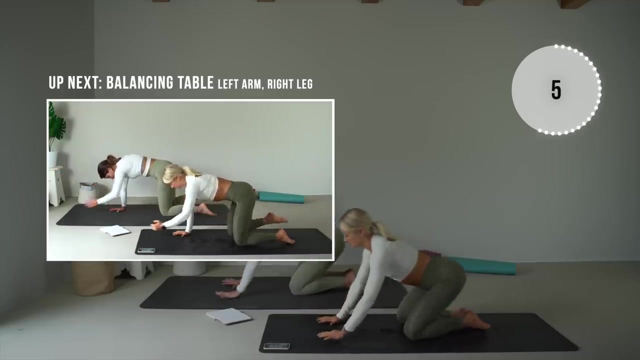 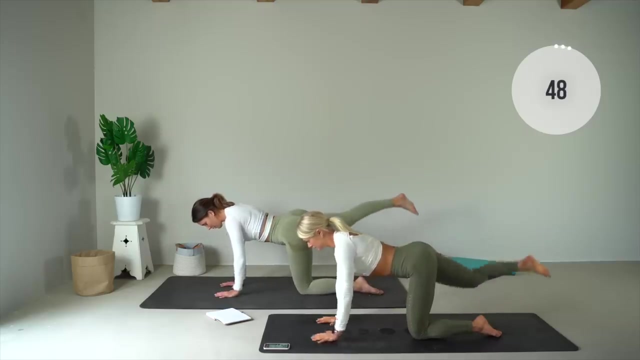 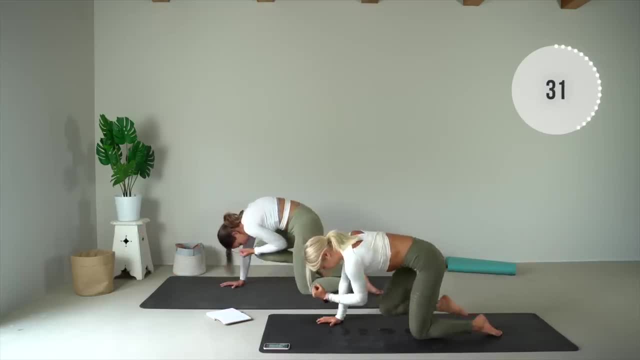 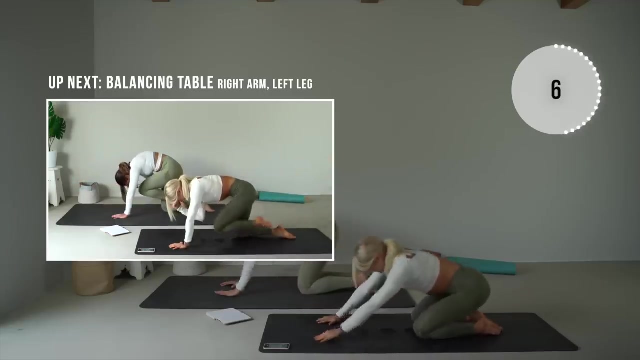 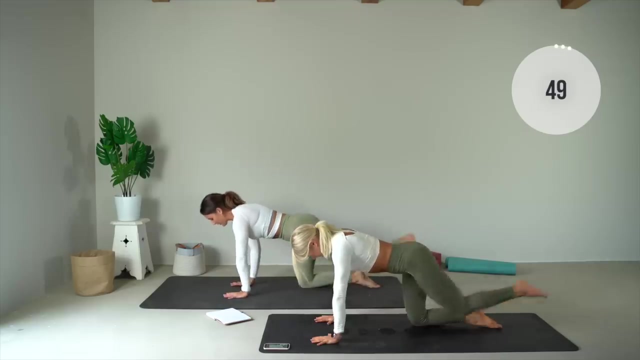 Thank you. First time I ever saw you, I fell in love when you entered the room And when the light hit your face. We were just kids, but I knew right away That I will be with you until I stop breathing. I will keep loving you as long as my heart speaks. 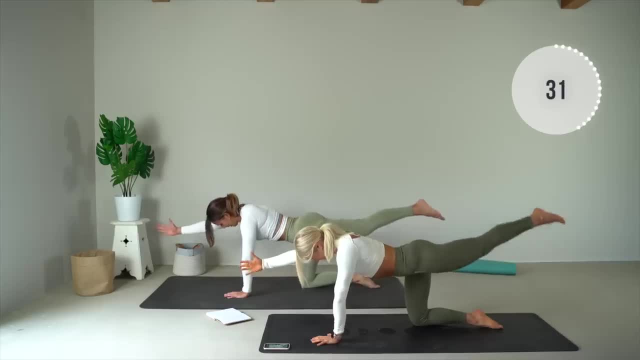 Oh, hold me close, Promise you won't let go. I'm nothing without you. I don't know what I would do without you. You are the one I choose. I wanna grow old with you. I'm nothing without you. I don't know what I would do without you. 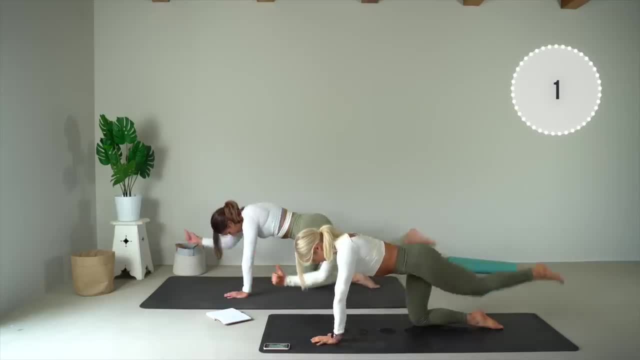 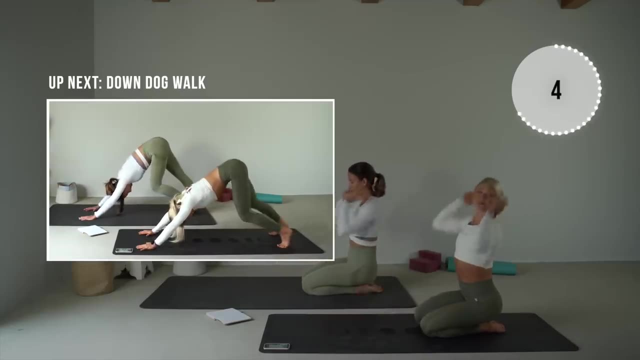 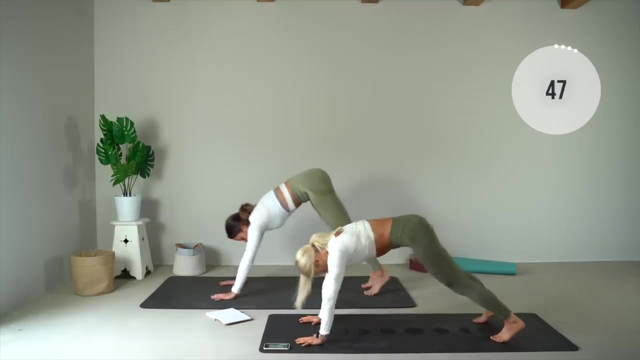 I don't know what I would do without you. I don't know what I would do without you. Even though years have gone by, I'm still in love with the way that you smile, And when I look in your eyes, I know that I will be with you the rest of my life. 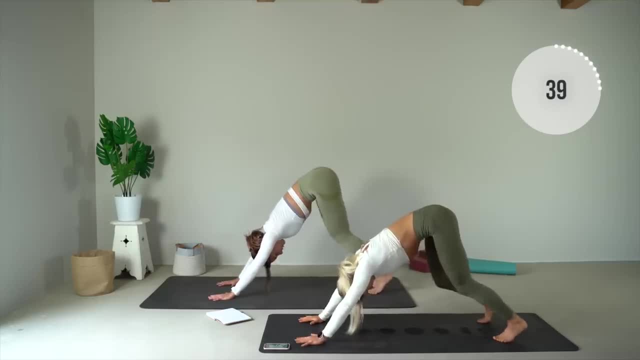 I will be with you until I stop breathing. I will keep loving you as long as my heart speaks. Oh, hold me close, Promise you won't let go. I'm nothing without you. I don't know what I would do without you. You are the one I choose. 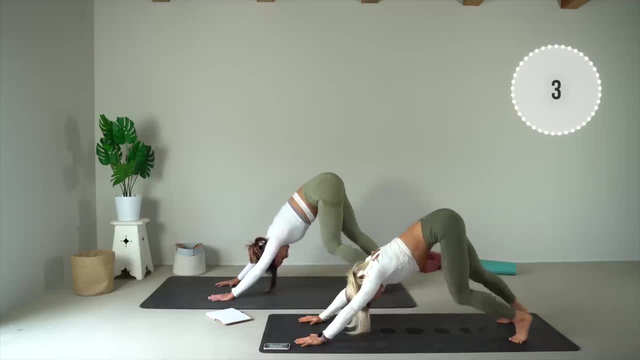 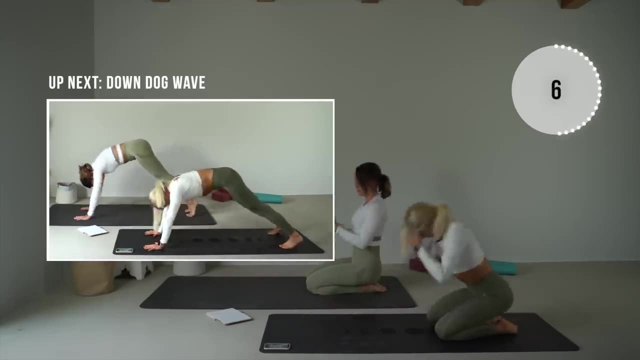 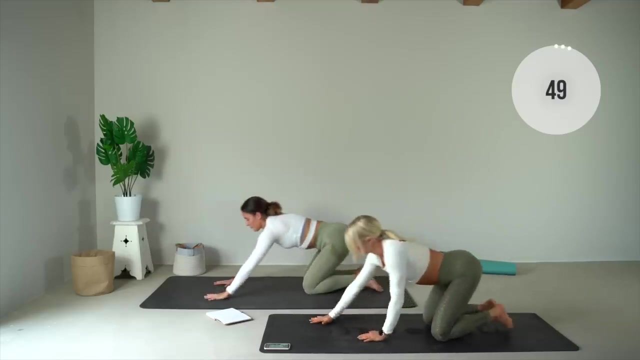 I wanna grow old with you. I'm nothing without you. I don't know what I would do without you. I won't let go. I'm nothing without you. I don't know what I would do without you. You are the one I choose. I won't let go. 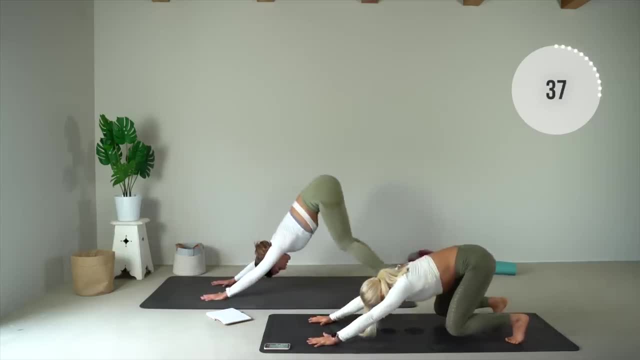 I'm nothing without you. You are the one I stay true to. Who was dancing all night With her stomachs full of butterflies? First time I saw her face, I fell in love. Oh, I can't believe you were mine. I'll never let you down. I'll never let you down. 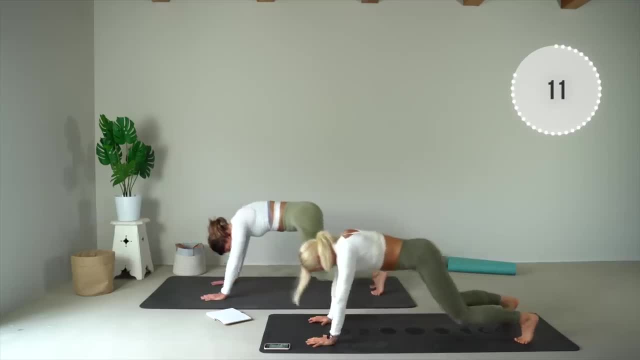 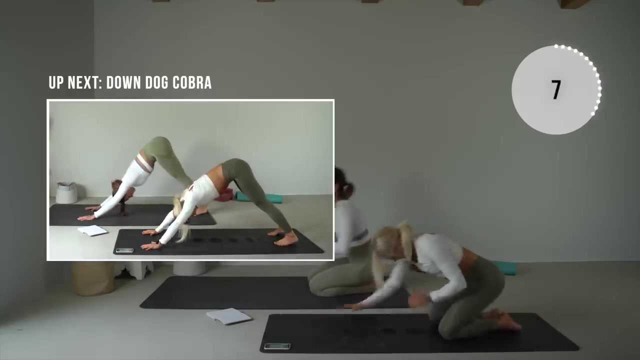 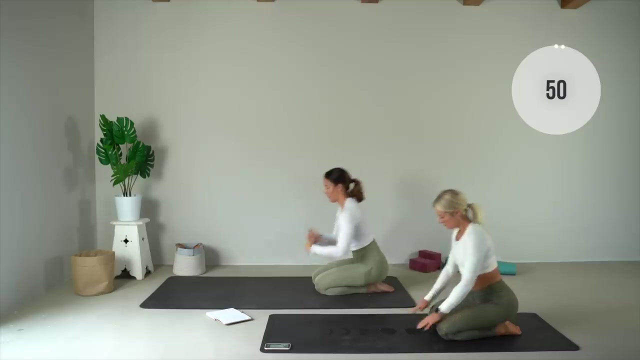 Oh, hold me close, Promise you won't let go. I'm nothing without ya. I don't know what I would do without you. You are the one I choose. I wanna grow up with you. I'm nothing without ya. I don't know what I would do without you. 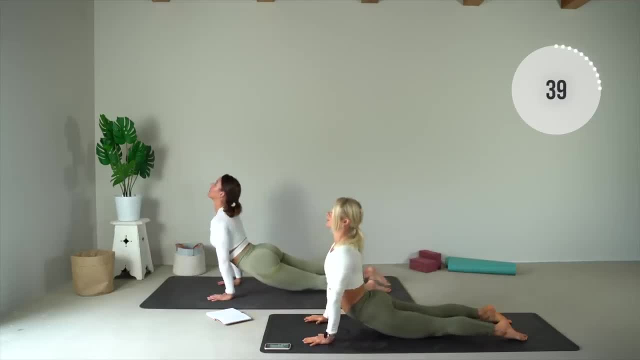 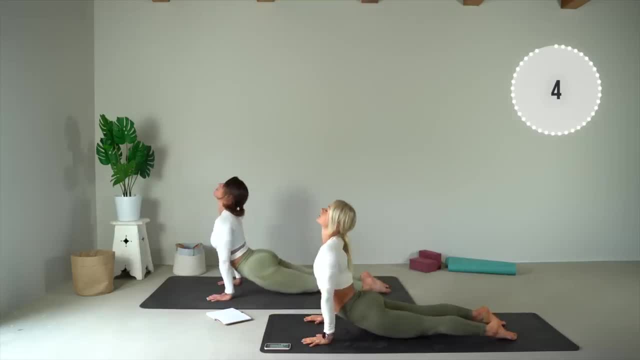 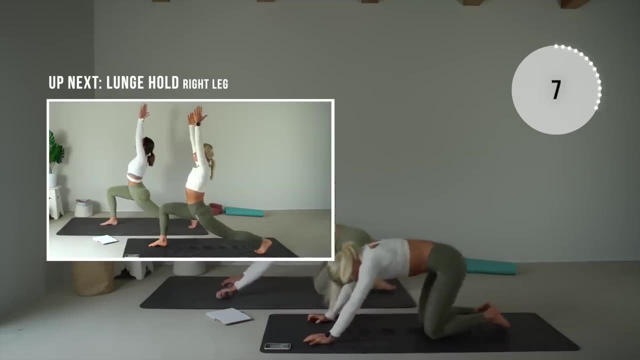 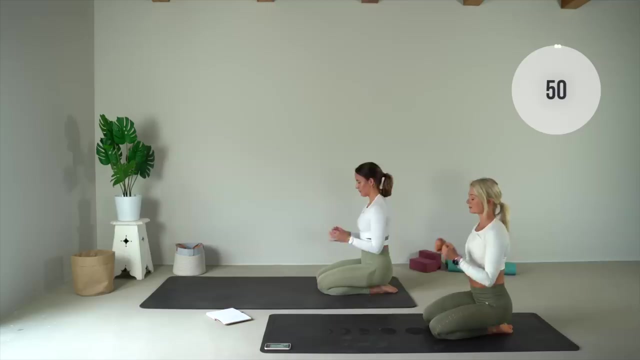 Do without you. I've been lying here for too long. I don't know what else to do. I wanna get away from every little thing. Just to try to make it through. I've been thinking about my options- Heavy detail in my head, But it doesn't really matter. 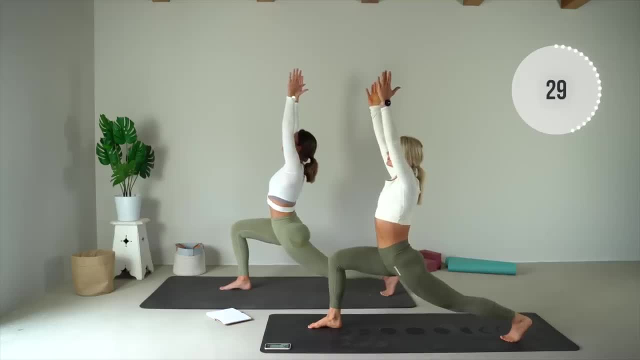 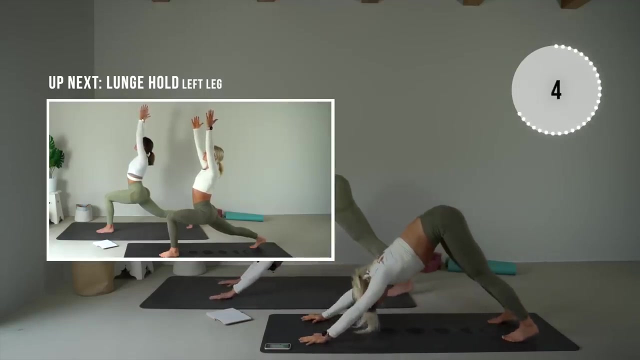 Nothing matters, so I cry instead. I've been running in circles Trying to catch my breath. I've been trying everything I can, But I ain't got nothing left. I've been staring at the ceiling. I've been staying up all night. Everything I ever worked for Vanished in the blink of an eye. 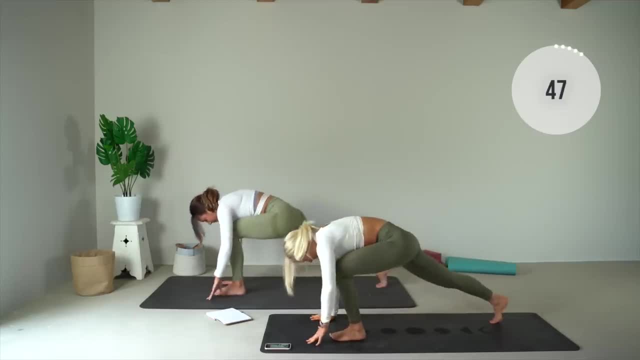 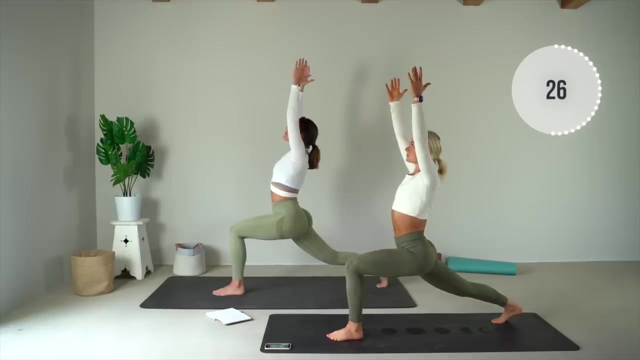 I've been asking every question Cause I haven't got a clue. Why's it gotta be me? What the hell am I supposed to do? I've been running in circles Trying to catch my breath. I've been trying everything I can, But I ain't got nothing left. 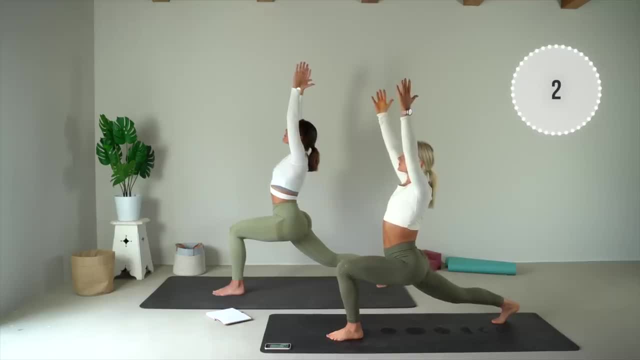 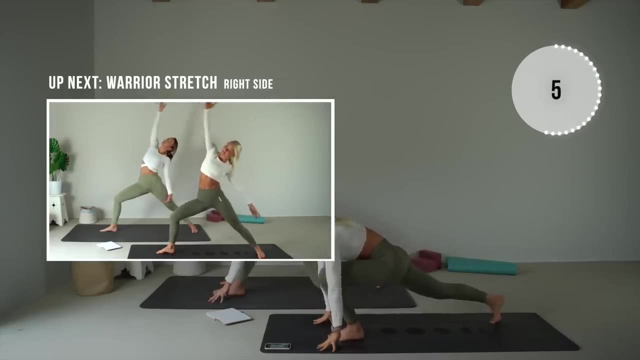 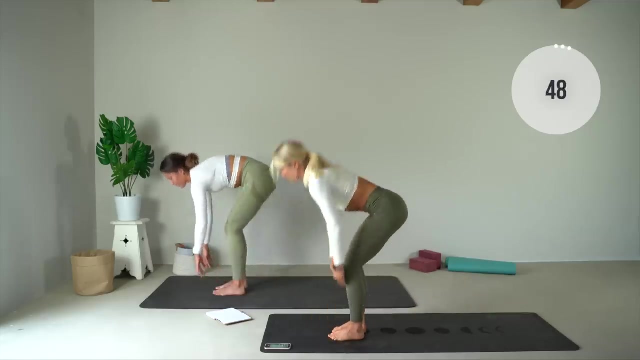 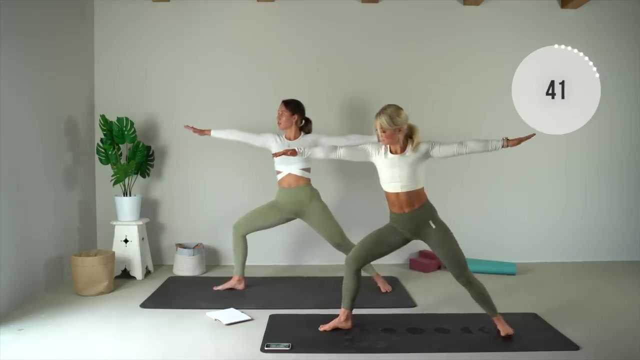 And I know there's so much more to this life, But it's hard to see it clearly. Yeah, I try my best, But nothing turns out right. God, I need you now so dearly, Cause I've been running in circles Trying to catch my breath. I've been trying everything I can. 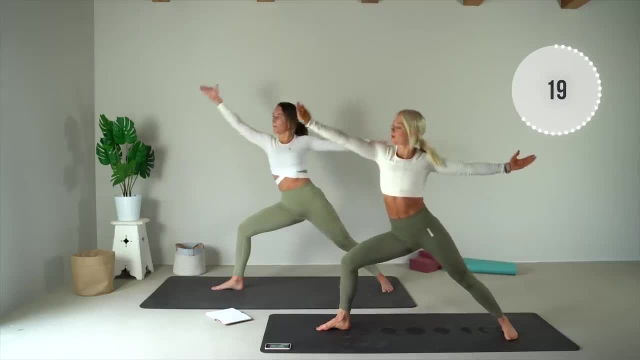 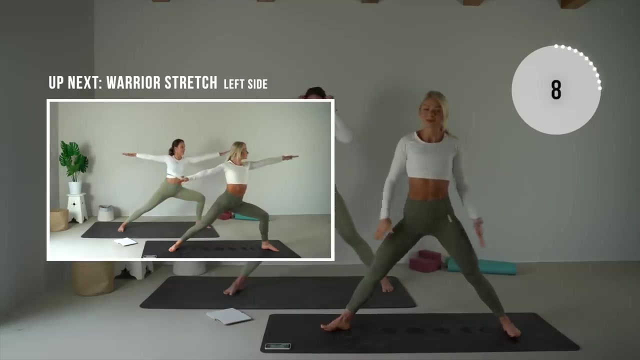 But I ain't got nothing left. I've been running in circles Trying to catch my breath. I've been trying everything I can, But I ain't got nothing left. I've been trying everything I can. I've been trying everything I can. I ain't got nothing left. 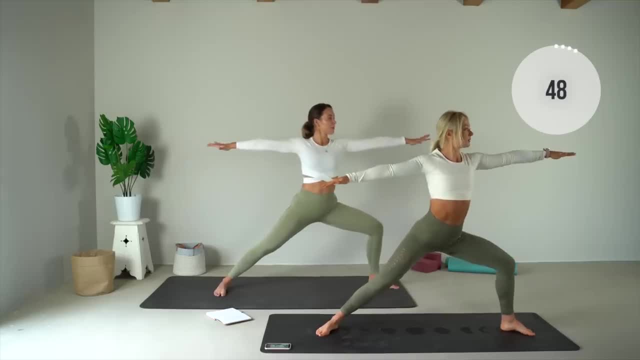 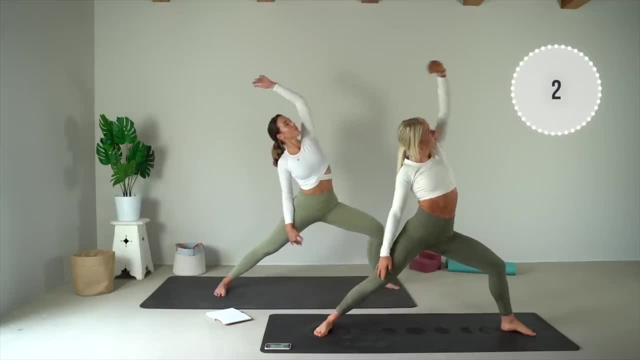 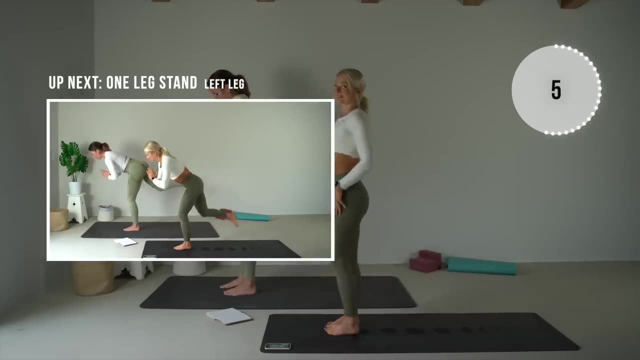 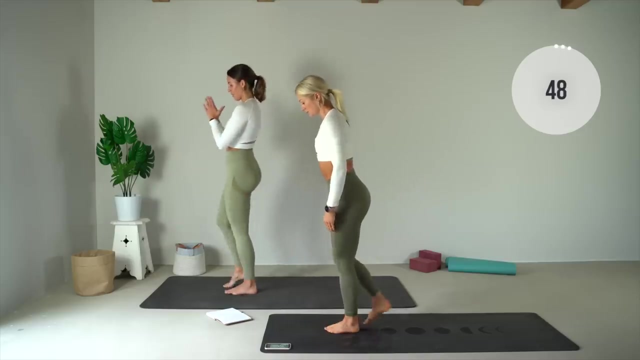 looks like you're changing and all, but why didn't you? why didn't you call something in the air? always something in the air. it explains: can you feel me? can you feel me? can you feel me? do you miss me at all? do you think about the things we used to do? 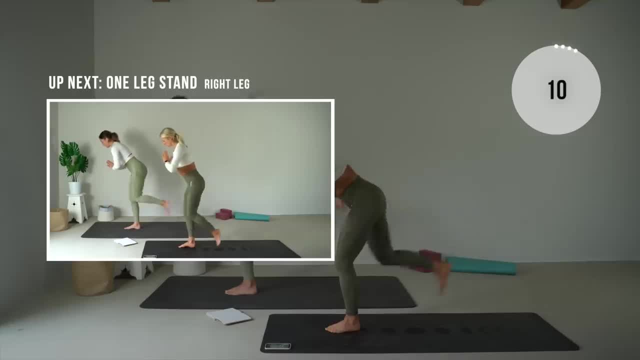 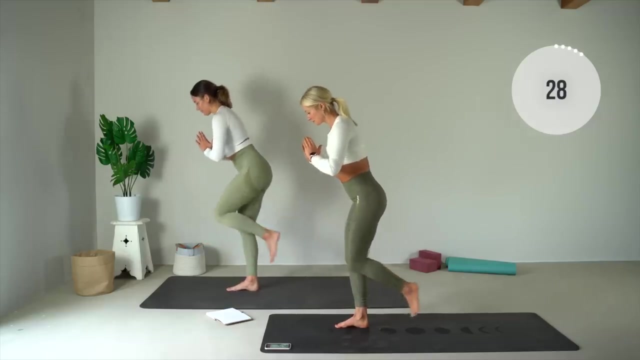 no, you couldn't stand tall. so why didn't you? why didn't you call? so many years it's gone by, but i think about you, about you all the time looks like you're changing and all. but why didn't you? why didn't you call something in the air, always something in the air. 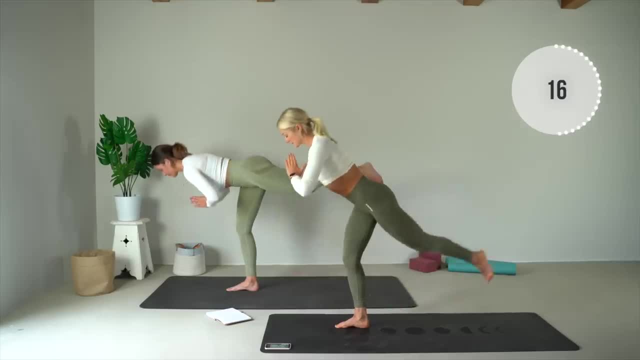 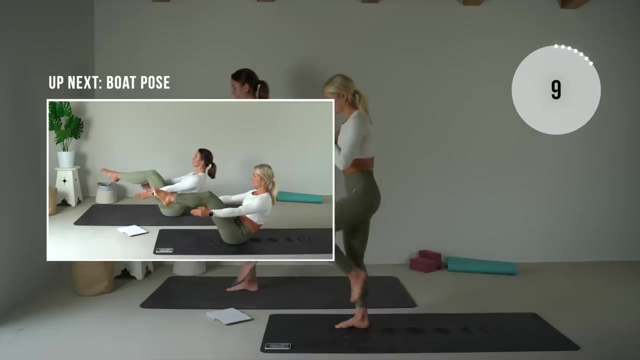 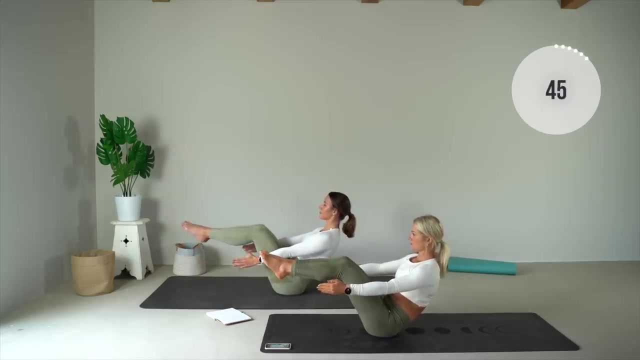 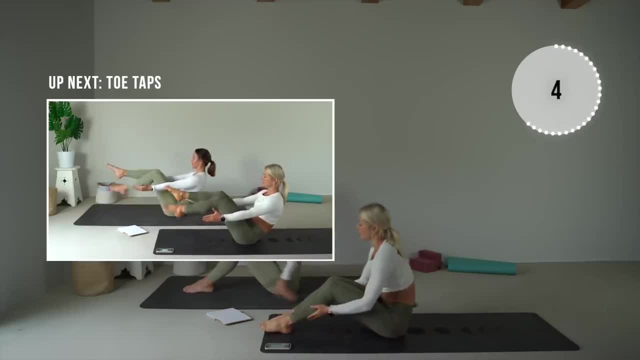 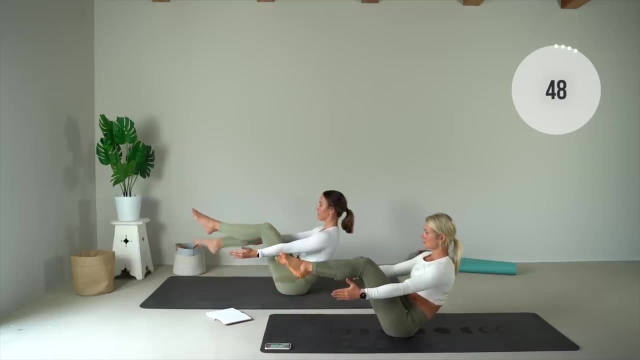 There's a new day to take away your sorrow. There's a new day to wash away the pain. Always get washed out by the rain. Darling, you've got to keep holding on through the night, Cause I promise you this If you try to get some sleep. 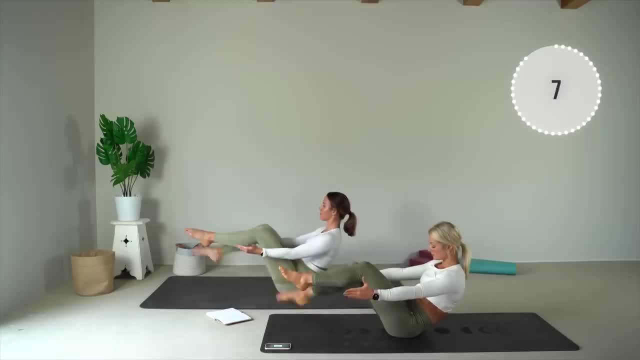 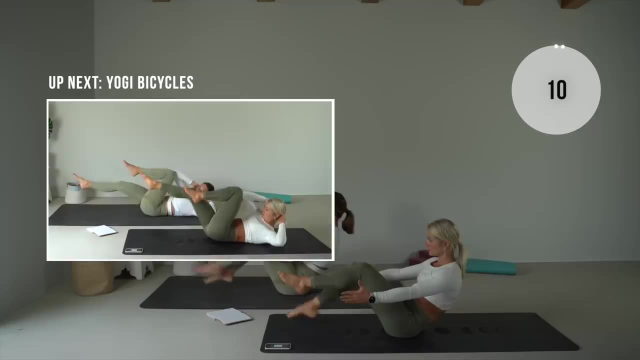 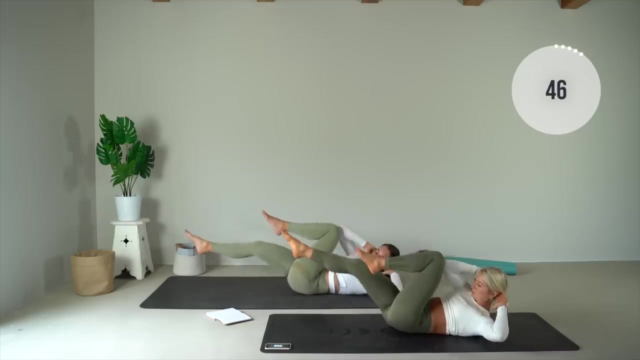 If you give up the fight, If only just for a bit. There's a new day to leave behind your troubles. There's a new day to wash away the pain. There's a new day and it will set you free. There's a new day to get you through your struggles. 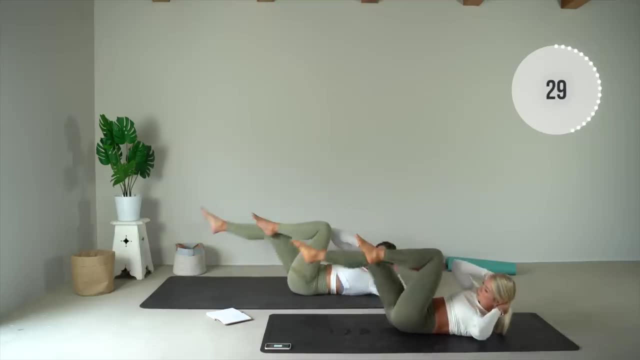 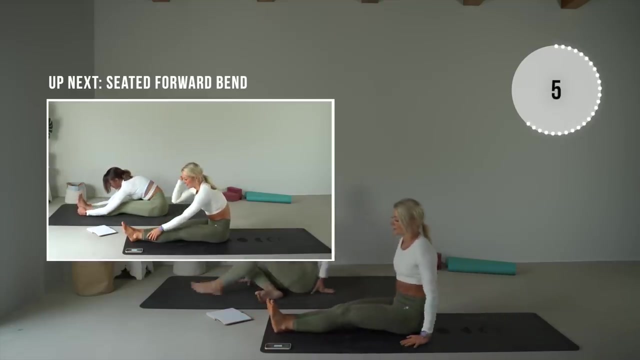 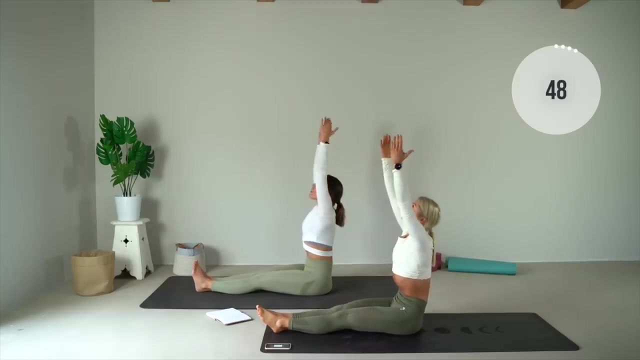 I will always think of you and me, Darling. You've got to keep holding on through the night, Cause I promise you this: If you try to get some sleep, If you give up the fight, If only just for a bit, There's a new day. It is waiting for us. 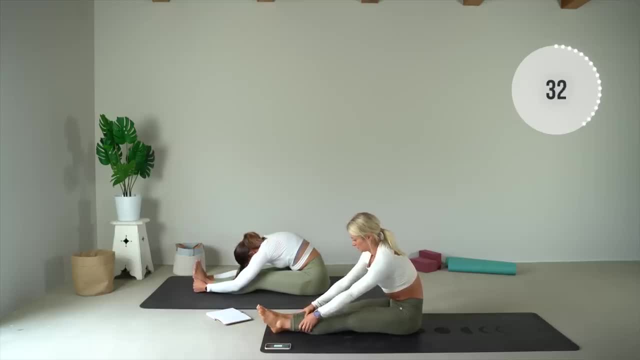 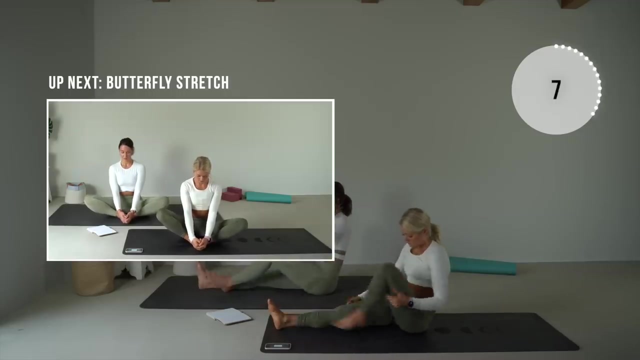 There's a new day Waiting round the bend. There's a new day, And it will restore us. And it will restore us Cause there will be new ways. This is not the end. Well, It'll still be the same. There will be new days. You'll probably 4 too. 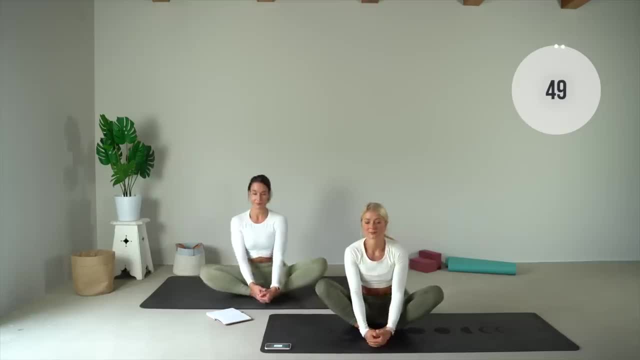 But we'll neglect you If you think you mean too much. Keep it on your mind. It's so hard to be near you. You make it hard for me to breathe And I can't stand to see you smile, Cause it kills me from within. Your voice is like an arrow. 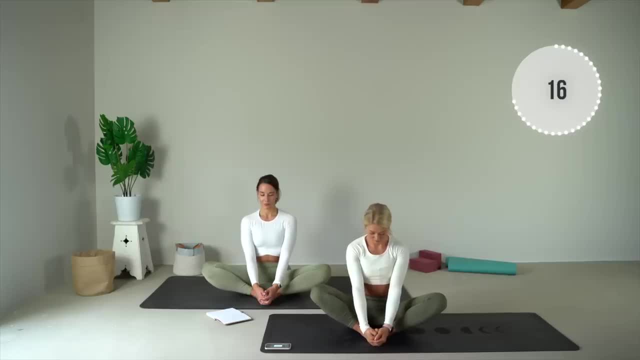 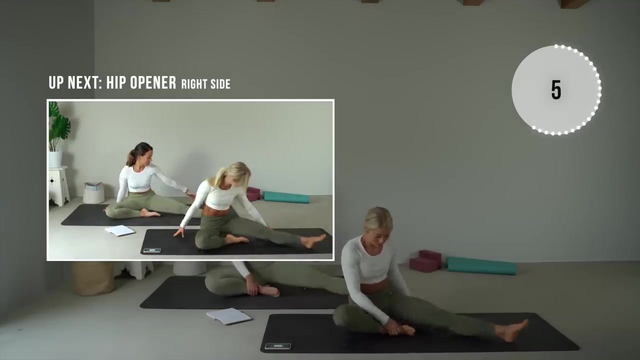 That pierces me through the heart, And your touch is like fire That will burn my skin. I wish that I could say What I really feel, Cause I'm in love And I can't stand to see you smile. And I can't stand to see you smile. 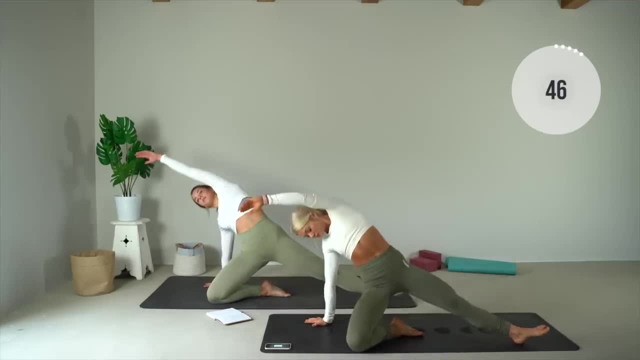 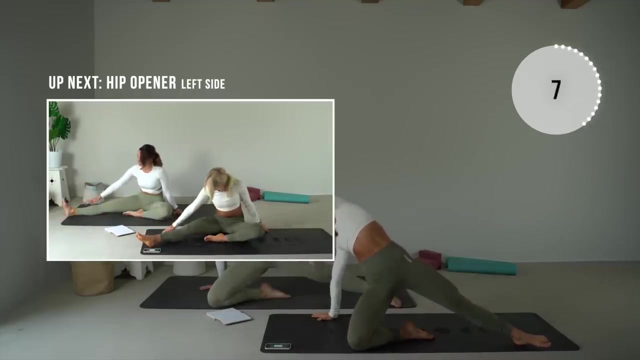 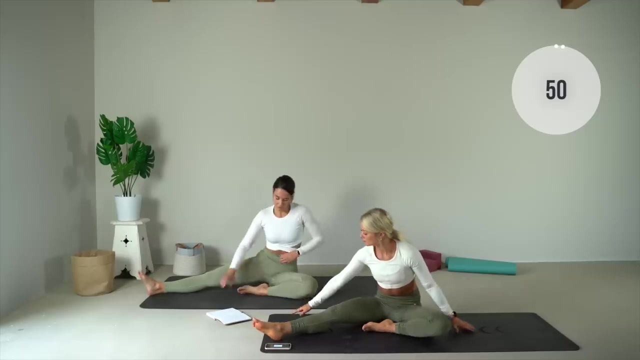 And I can't stand to see you smile. It's so hard to see you When you are with him. It's so hard to hear you When he makes you laugh. The ring around your finger Is a noose around my neck And I can't stand to see you smile. 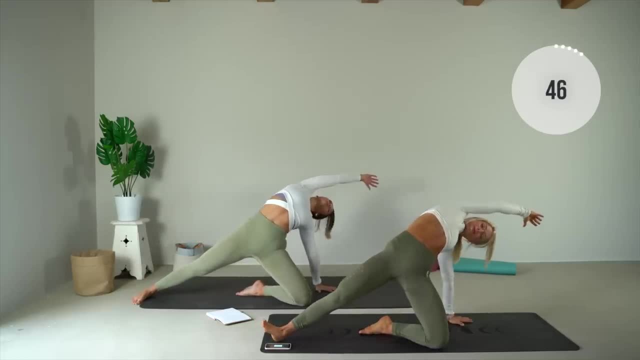 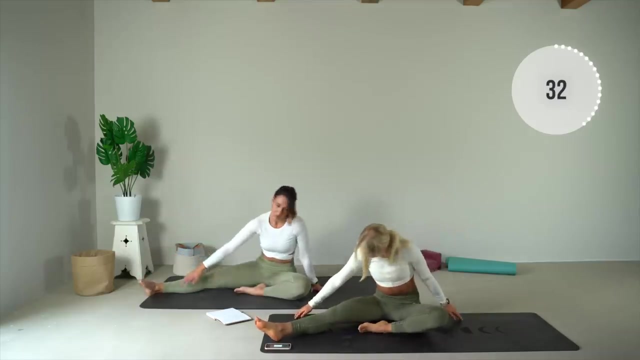 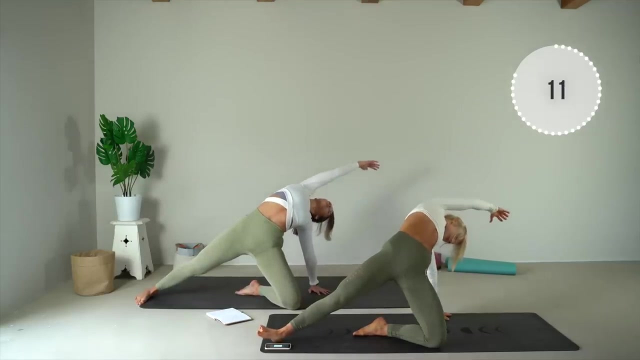 I tighten with every hour And every day that passes by. If only you could see That it should be you and me, Cause I'm in love with you. Yeah, I'm in love with you. I'm in love with you. I know I'm not supposed to be. 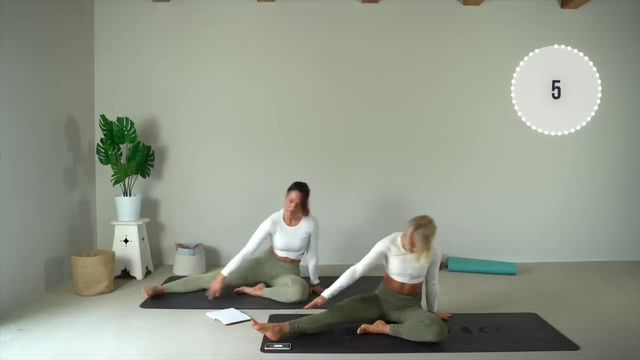 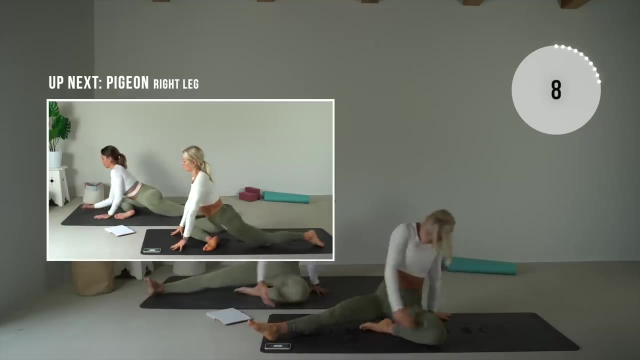 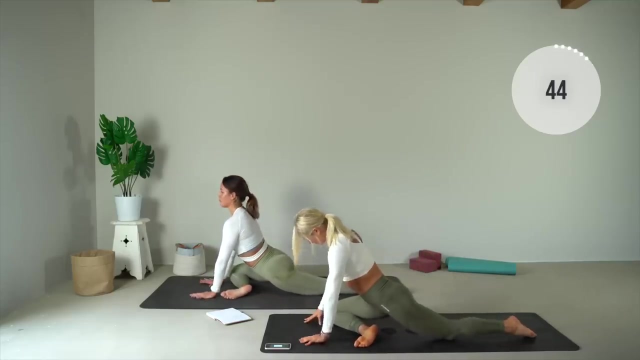 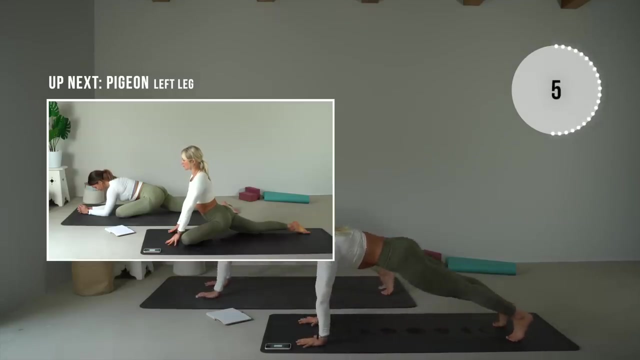 But I am, I'm in love with you. Yeah, I'm in love with you. Yeah, I'm in love with you. And sauce from your lips? Yeah, I'm in love with you. Oh, I want you to know. Thank you, Thank you. 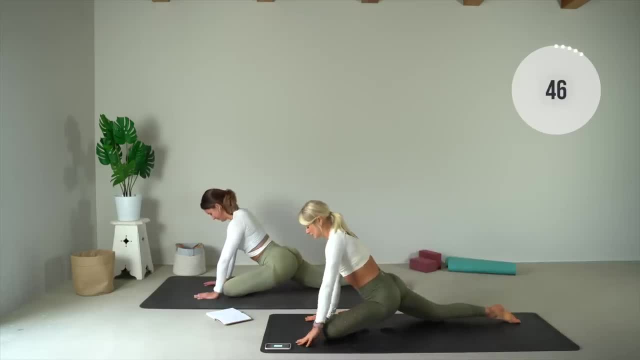 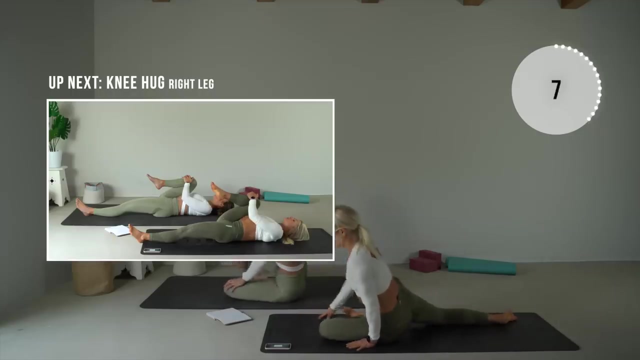 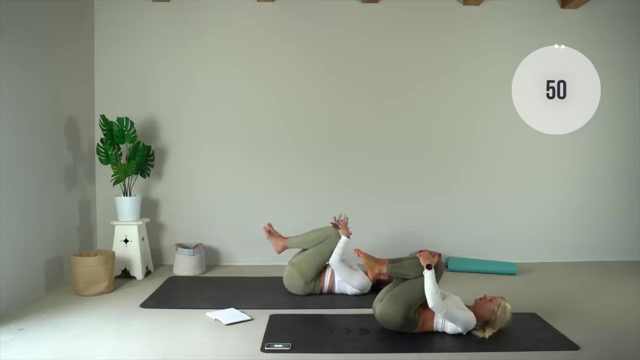 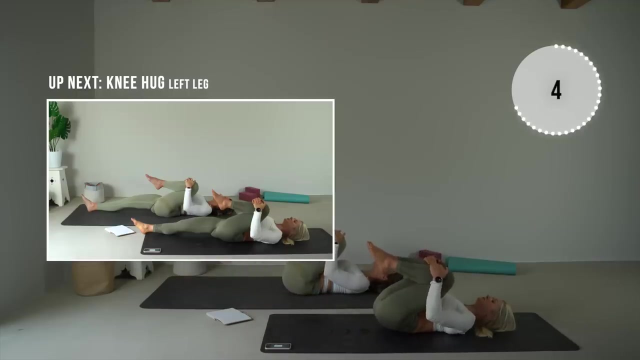 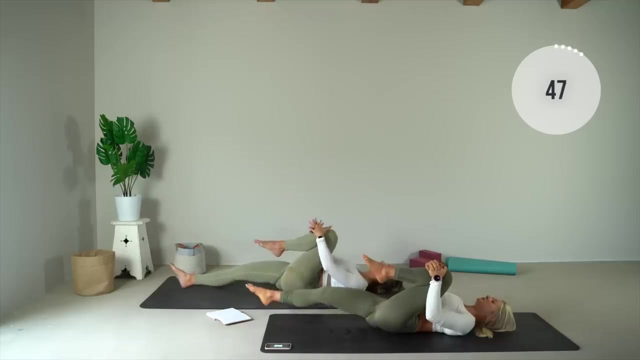 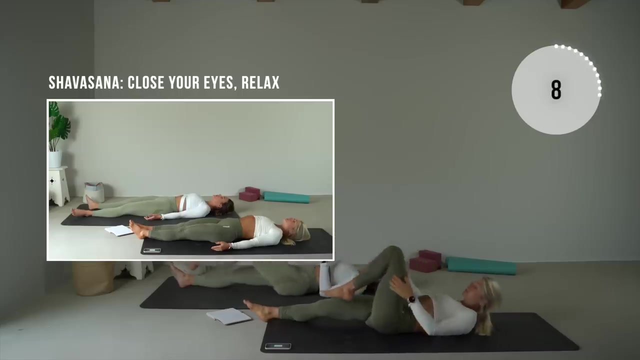 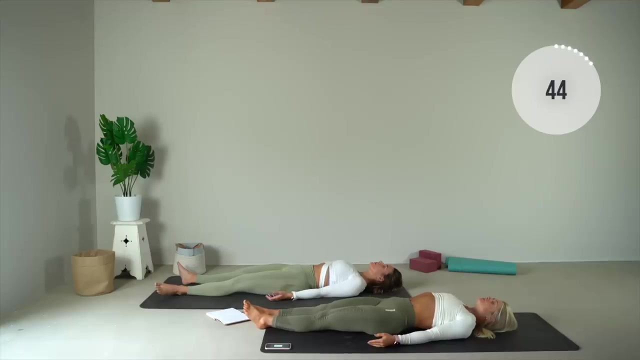